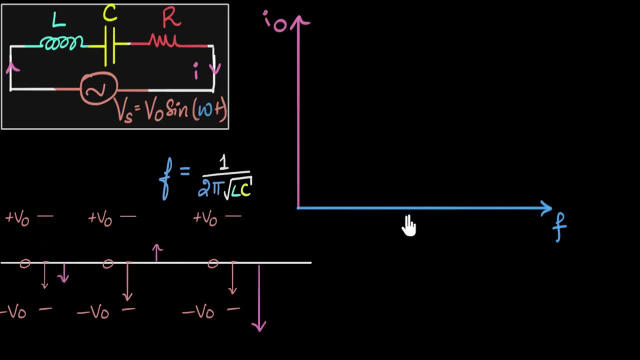 Now, before I draw it, I want you to take a shot at this. One clue is that we know that at resonant frequency, the current is maximum, So let's assume that that resonant frequency is somewhere over here. So, given that we know that at resonant frequency, 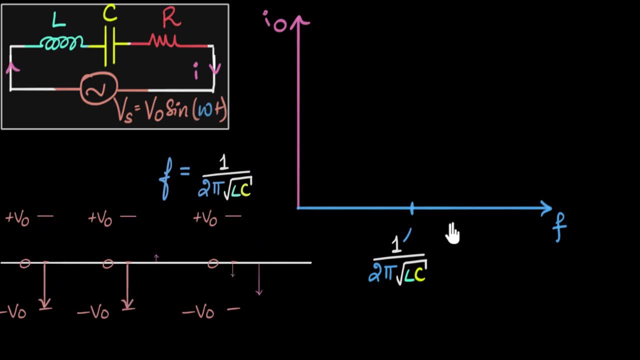 the current is maximum, So let's assume that that resonant frequency is somewhere over here. So, given that, can you make a guess as to what this graph would look like? Go ahead, give it a shot. All right, if you're giving it a shot, let's see. 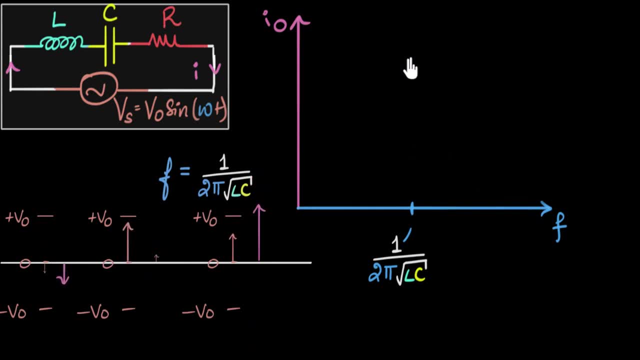 Here's how I'm thinking. I know that at this point my current has to be maximum, Which means if I go away from here, on either sides the current should decrease. So with that, if we plot the graph, here's the maximum. 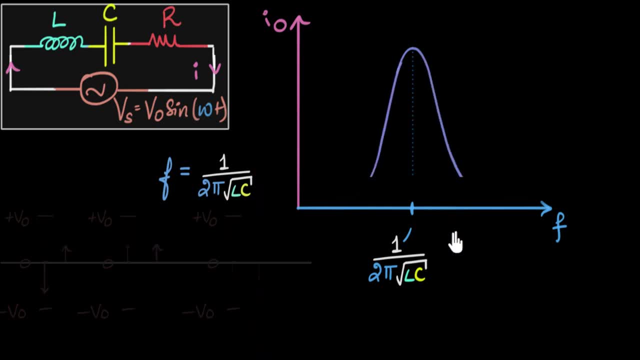 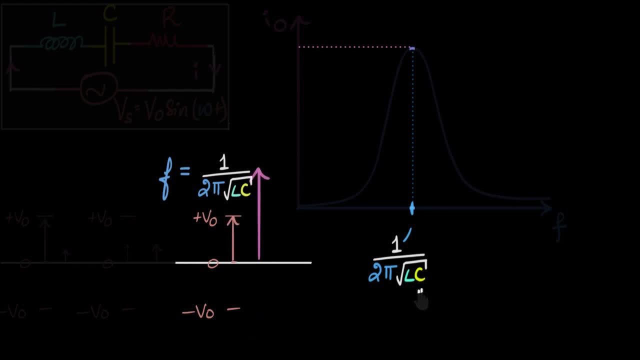 And on either sides, the current decreases, decreases, and that's what the graph would look like. Again, notice: it's telling us the same story At resonant frequency. the current is maximum, But if you go away from it with too low, 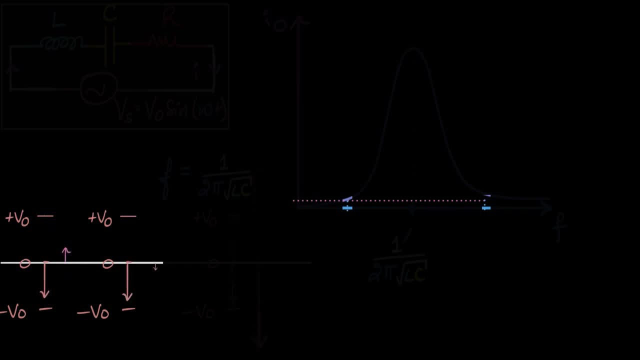 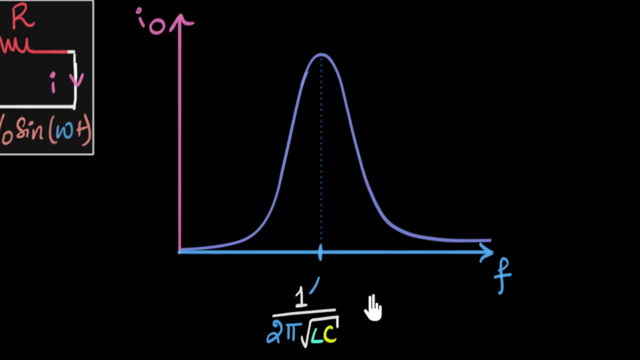 or too high frequency. then notice, the current becomes minimum, So we can get rid of this animation. We can now just focus on this graph. Okay, now with this graph, let's see if we can decipher the mysteries of radio, The important thing to understand. 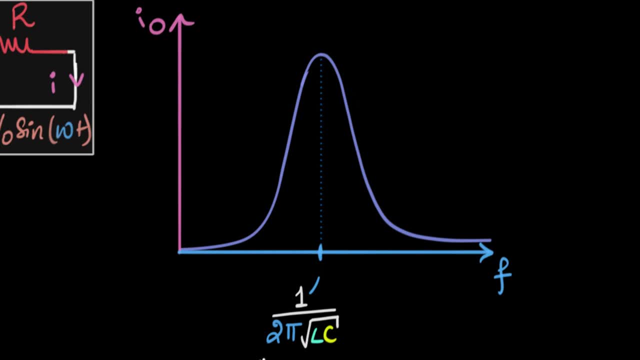 is that different, different radio stations get broadcasted at different frequencies. For example, just name a couple of famous radio stations that I am aware of. I know one radio station called Radio Mirchi, and all the messages over here gets broadcasted at 98.3. 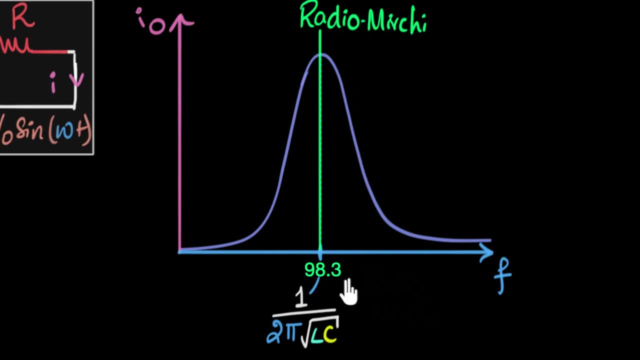 and that's why you may have heard this number a lot: 98.3 megahertz of frequency. So whenever you're listening to Radio Mirchi, or if you want to, then that is at frequency of 98.3 megahertz. 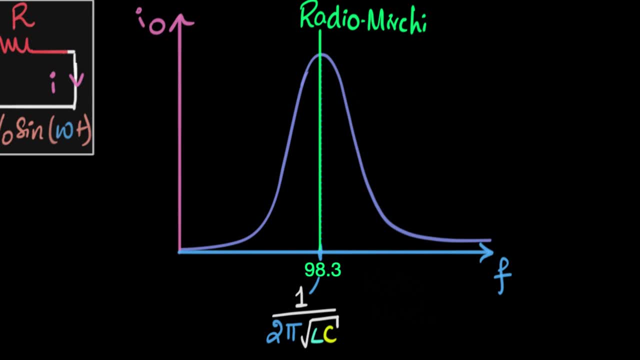 Similarly. let me just show one more. Another one which I remember is Big FM, and again they have that punchline 92.7 Big FM and that basically means they are broadcasting all their messages at 92.7 megahertz. Now let's imagine that in our radio currently. 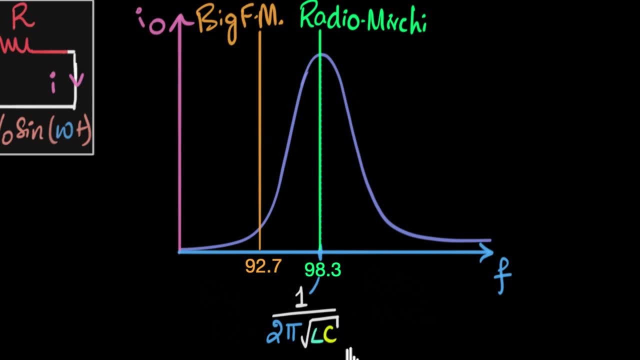 the LC values are such that if you calculate the resonant frequency, it happens to be exactly 98.3 megahertz. Let's assume that What's gonna happen? Well, here's our radio, and here are both the radio waves I've shown. 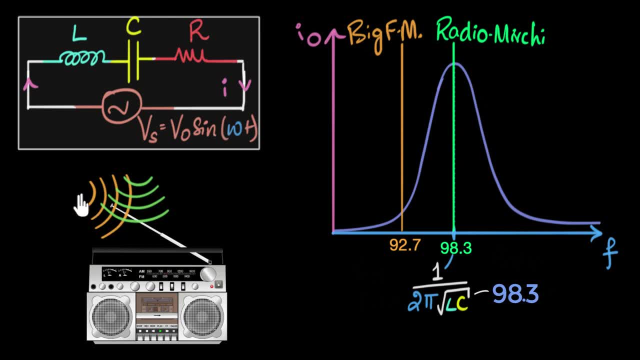 There are multiple radio waves due to lots of channels, but let's assume just two. They're both hitting our antenna and, as a result, antenna vibrates with both the frequencies. What an antenna does is basically converts radio signals into electrical signals. So because of these two 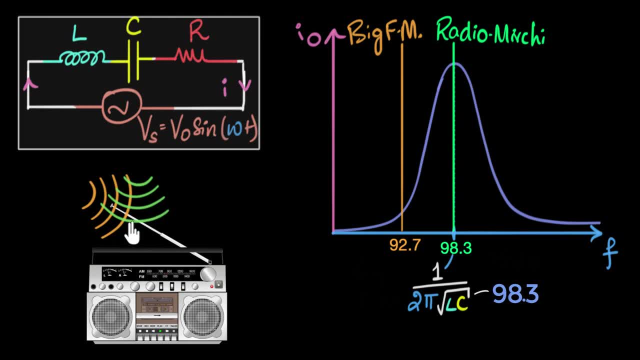 the antenna is trying to drive our LCR circuit at both these frequencies. But look from the graph. we can see that whatever messages are coming at 98.3, it's able to generate a much larger current. Let me show you that. 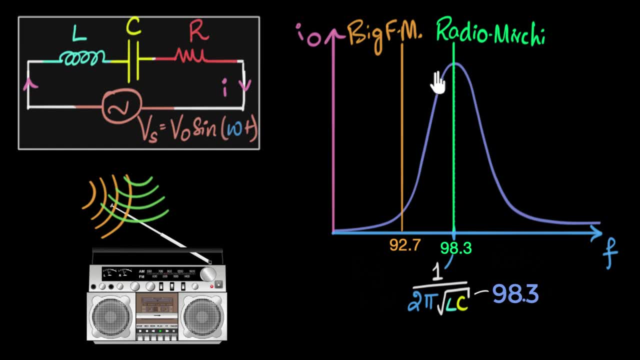 It's able to generate a much larger current. The current that that is generating is over here due to the radio Mirchi signals And the current that is generated due to the Big FM. look at that. That current generated is very tiny And, as a result, this very high current goes through the speak. 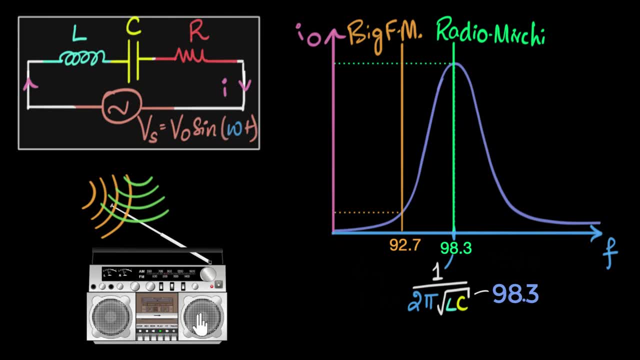 And this current? well, it can hardly drive the speaker And, as a result, you will only hear the messages from this particular channel. Now imagine you want to switch to Big FM. What should you do? I think you can now guess. 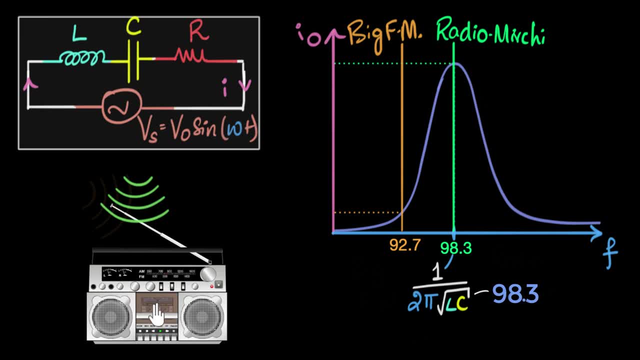 Well, now we need to reduce the resonant frequency of our LCR circuit. How do we do that? Well, you have to either. now, since you want to reduce this, we need to increase this. So you either increase the inductance. 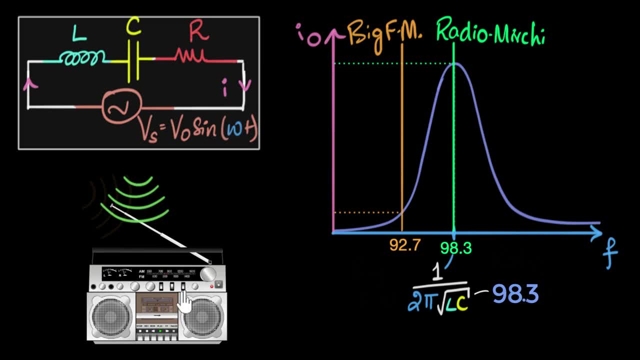 or you increase the capacitance, And there are ways in which it can be done. Different radios do different ways. For example, in some radios, when you turn the knob, the distance between the plates of the capacitor changes And you might know as that distance changes. 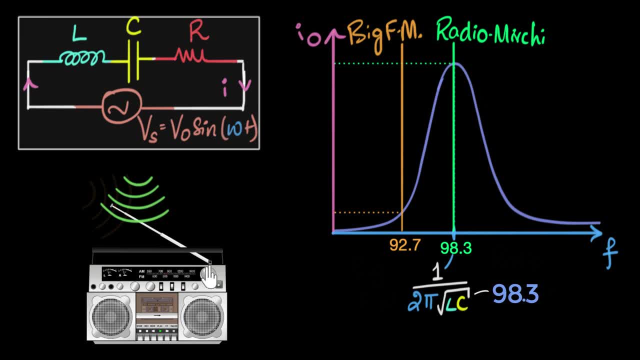 the capacitance changes- Interesting, isn't it? And so, just by turning the knob, one of them will change, And in this particular case, all we have to do is increase the value of capacitor. And as you increase the value of capacitance, 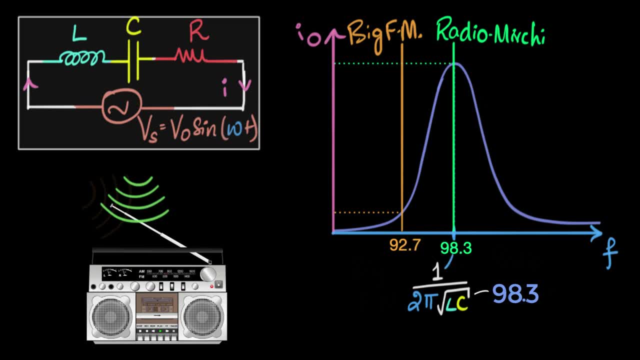 the resonant frequency will start shifting towards the left, So the graph will start shifting towards the left, And so your new graph. as you increase the value of that capacitance, your new graph will eventually come to this. Now the opposite happens. 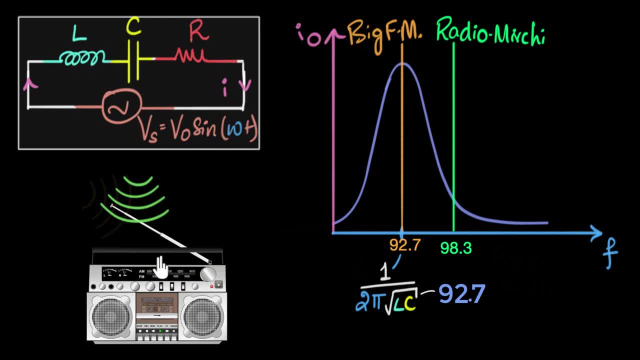 Now it's the Big FM. It's these messages that start exciting your radio, because your radio's resonant frequency has changed And, as a result, your radio will start picking up those signals. And this is how, by using resonant frequency concept. 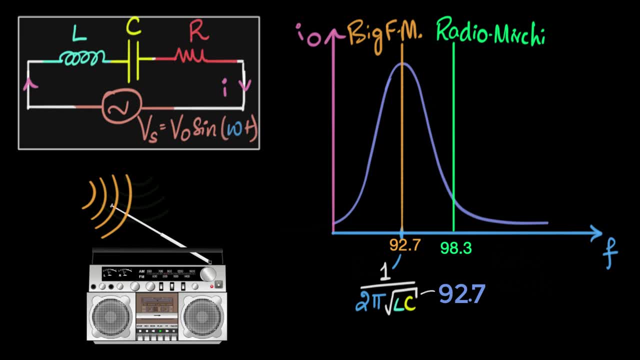 resonance concept. you can tune into any station that you want. Beautiful, isn't it All right? now let's make things a little bit more interesting. Imagine your friend also has her own radio, And let's assume, for the sake of simplicity, 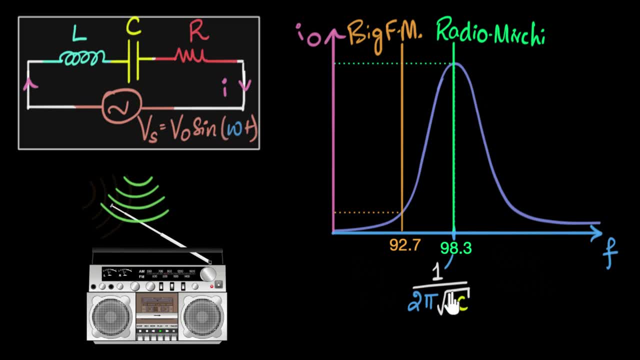 that in her radio the value of inductor and the capacitor, as of now, is exactly the same. So it's resonating at 98.3 megahertz. But there's one difference. Let's say that the resistor, the resistance of her LCR circuit, 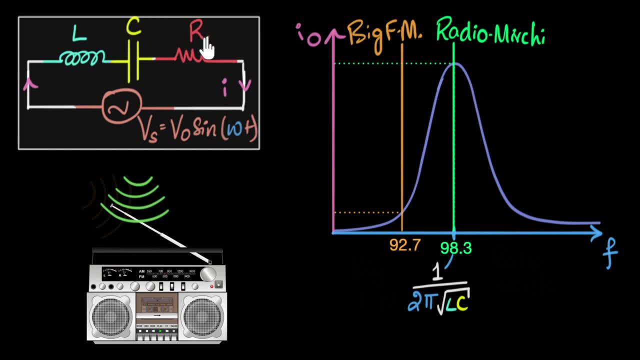 is higher than your LCR circuit's resistance, So the value of resistance is higher. I want you to predict what that new graph of this new radio is gonna look like: Same resonant frequency, but higher resistance Again. can you pause the video and give this a shot? 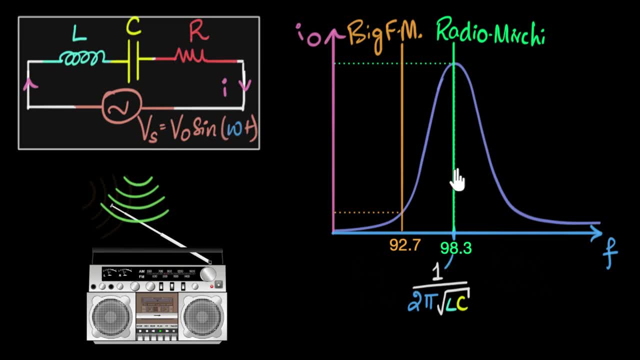 All right, because it has the same resonating frequency, it'll peak at the same frequency. However, at the peak value, the current would be smaller because the resistance is higher, And so the graph that we could expect is somewhat like this. 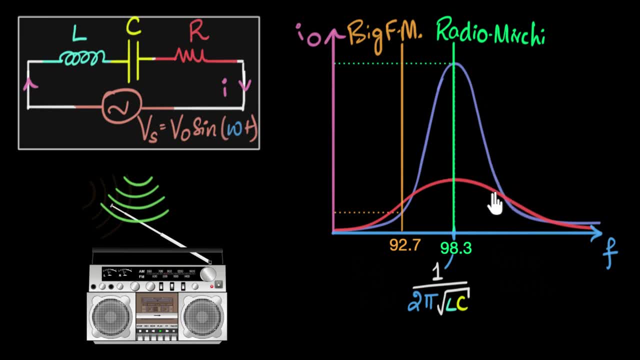 You immediately see the graph is much flatter than before, and that has consequences, For example, if you just concentrate on this graph. so let me just get rid of the other one and now look at what's gonna happen to the radio. Just like before, this frequency is gonna. 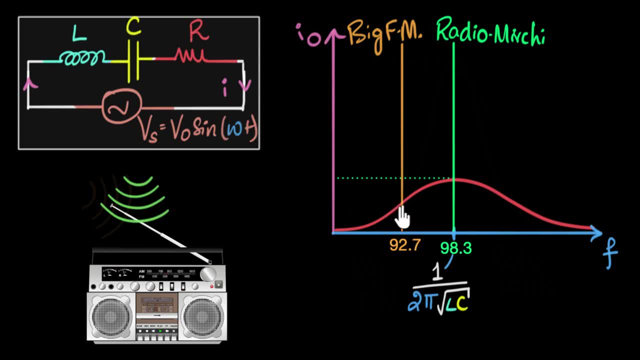 generate the maximum current. but notice, because the graph's like this, it will be backgrounding. All right. now, that's it. I just can't hear you because the graph is so flat. the current generated by the big FM frequency. 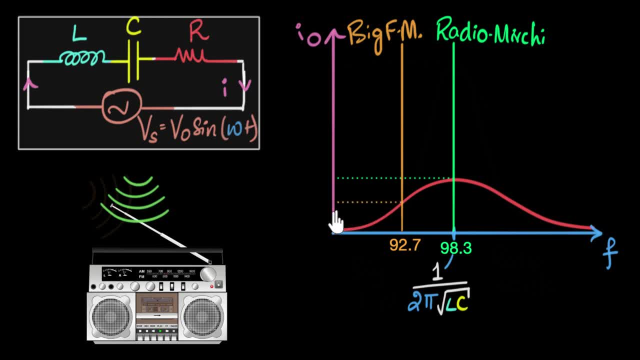 is considerable. It is smaller but it's considerable, Which means, in this particular case, your radio might be giving some amount of message from this as well. There will be some mixed messages that you'll be getting. You'll be able to hear this.